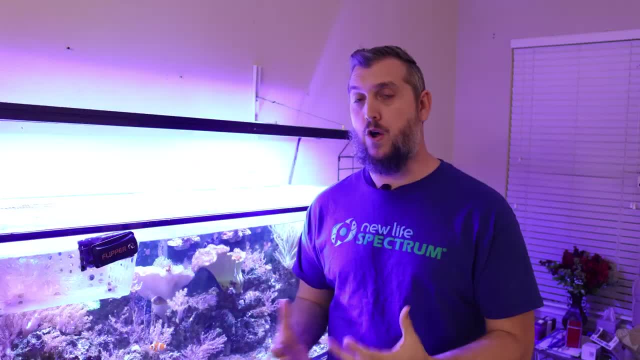 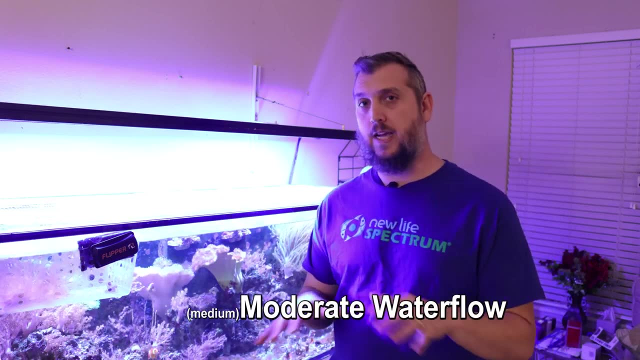 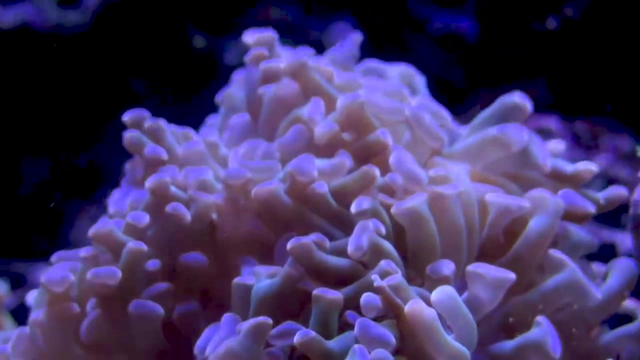 can see them moving around. There's not no flow where they're just kind of sitting there. You want to add some motion through your coral. So medium flow is kind of a good place for euphelia. Some do really well in a lower flow too. They just don't like to be blasted with a lot of. 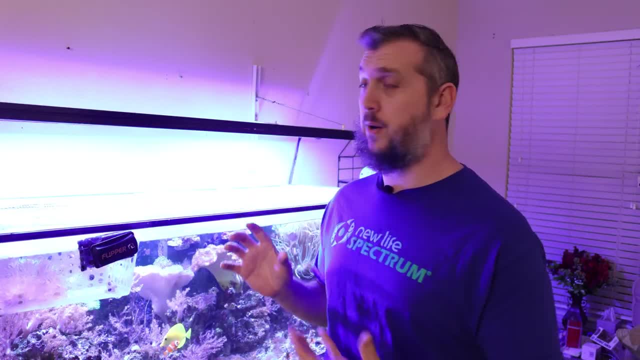 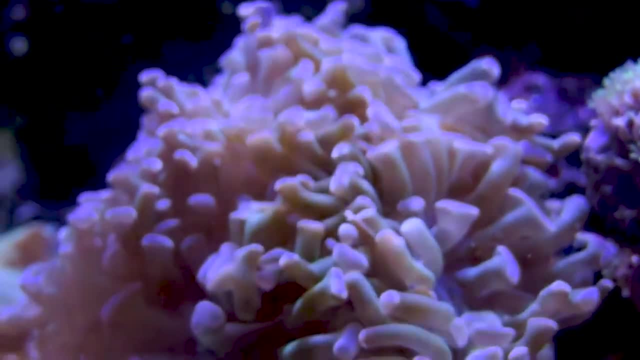 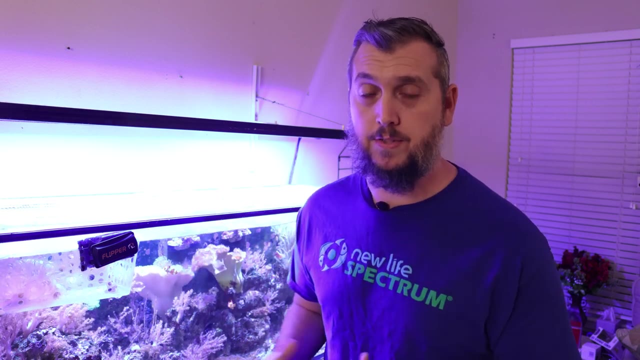 flow. So you don't want to put them directly in front of your powerhead or circulation pump in your tank because that would be constant water flow, just blasting the coral, And you can push too much water into the coral and make them recede or even take the tentacles right off of the. 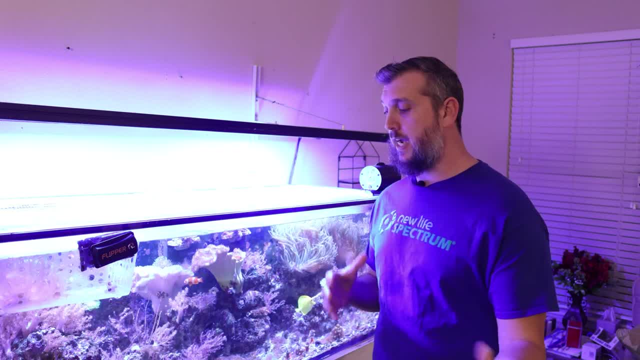 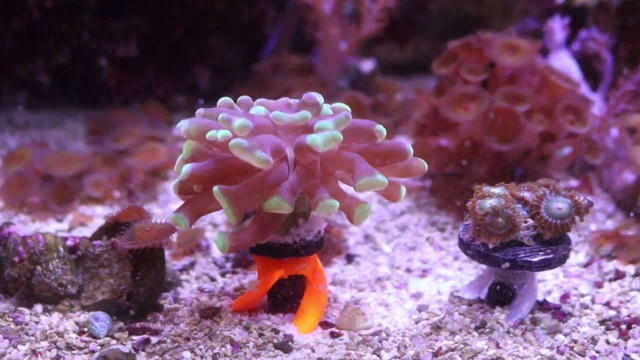 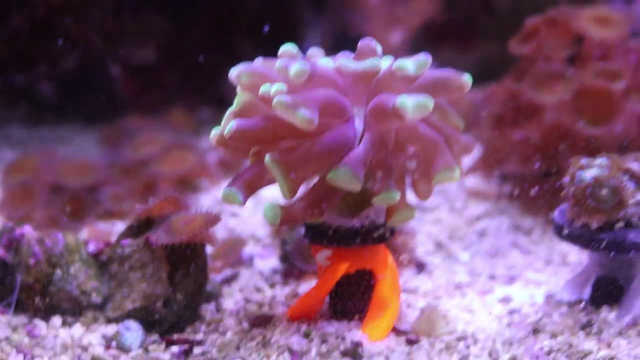 skeleton. So we don't want to do flow like that, Just a nice easygoing flow through your coral, nothing too turbulent. So I just recently added a hammer coral to this aquarium. So, for example, I'm using one of the Printed Reef sand stands to kind of. 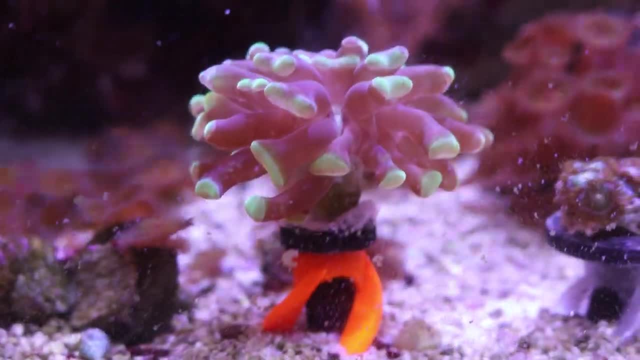 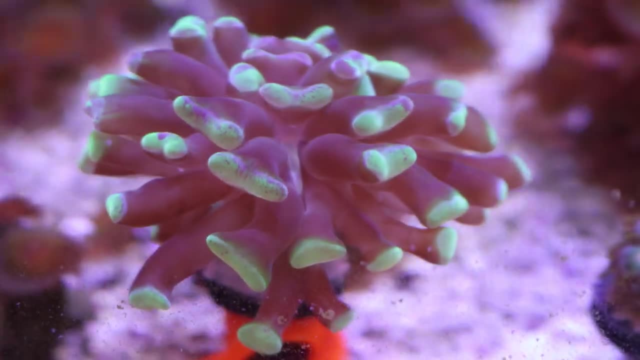 hold it down in place and keep it low on the sand bed first. Now these 3D printed products help keep your corals safe while they're sitting in the sand bed, while you're getting them acclimated and adjusted to your aquarium. It's also worth mentioning in the beginning that you don't 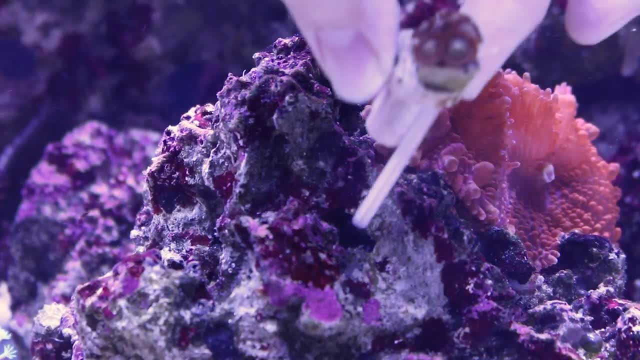 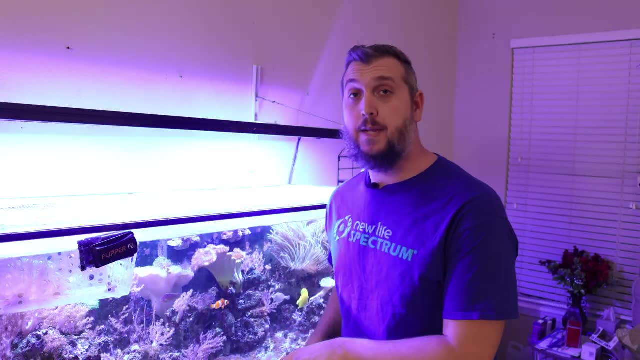 necessarily need to glue your coral frags down and put them in a permanent home right away. Now it's a good idea to introduce any new corals at the bottom of your aquarium. put them on the sand bed. You don't necessarily need to start them high up on the rock work or in. 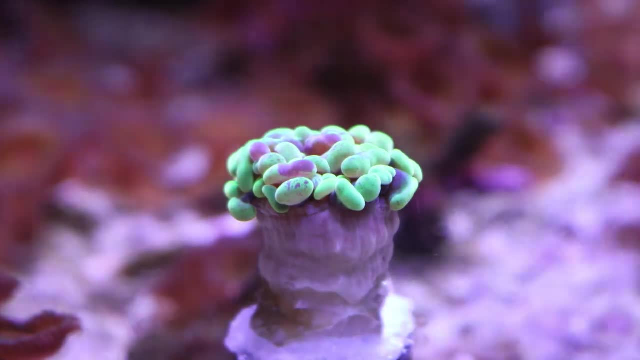 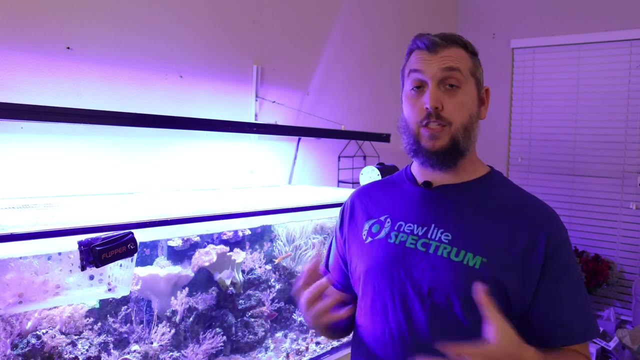 the middle of the rock work because you want to slowly adjust them over time. So when you put them in your tank you can let them sit a few days to a week, monitor how they're doing, how they're adapting and getting adjusted to your tank, and then you can move them up from there. So things 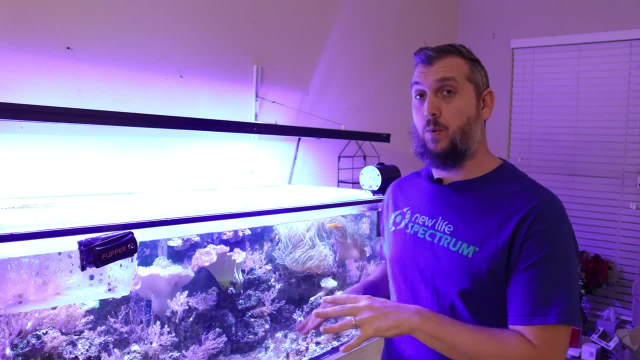 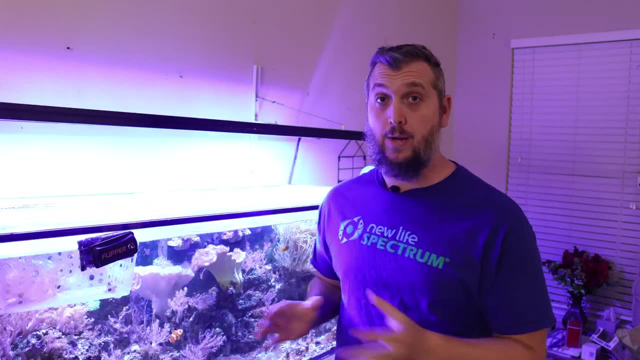 like Acropora, usually like it high up in the rock work and they like higher lighting. Acropora is SPS coral and that stands for for small polyp stony coral. now hammer corals are lps corals and that stands for large polyp stony. 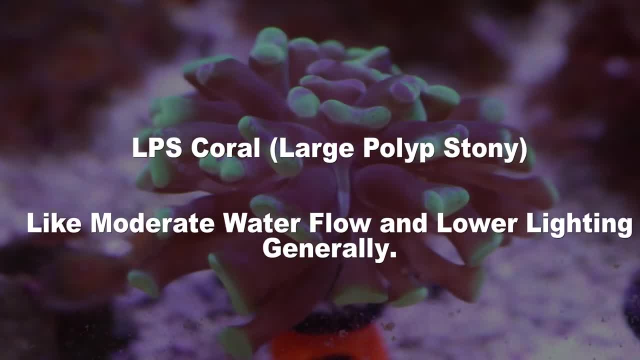 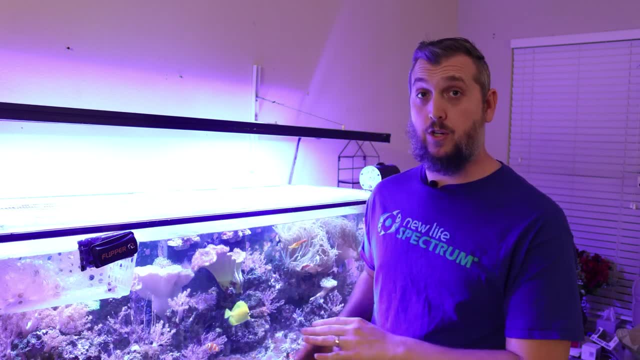 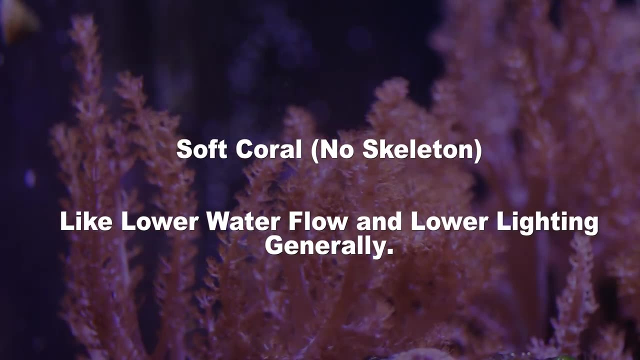 corals because they have that large fleshy tentacles to them so they can be medium to low in your aquarium. but when you first put them in your tank, make sure you start them on the bottom and slowly get them adjusted now something like a zoanthid or a kenya tree. coral is a soft coral.